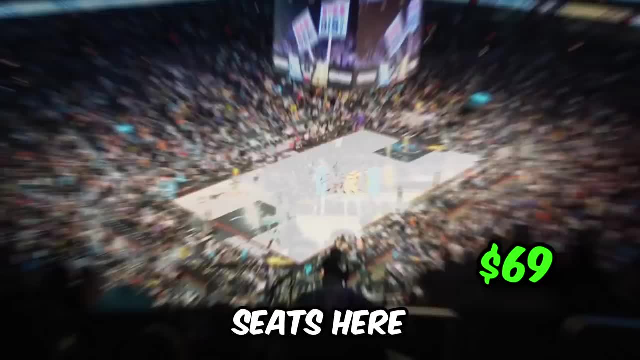 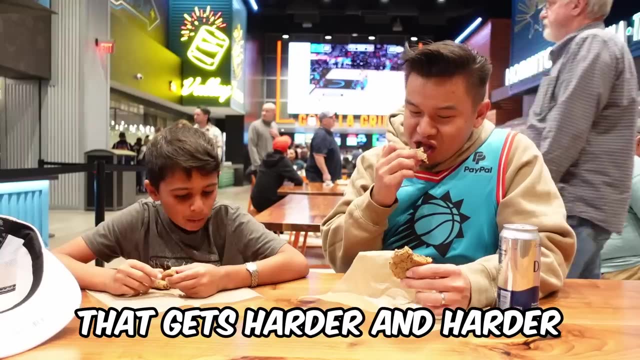 I am at the Suns Footprint Arena and I bought the cheapest seats here to the most expensive seats. here We have seven NBA seats that get better and better. Each seat will have a challenge that gets harder and harder, but the seats will get more and more expensive. Eventually we'll be 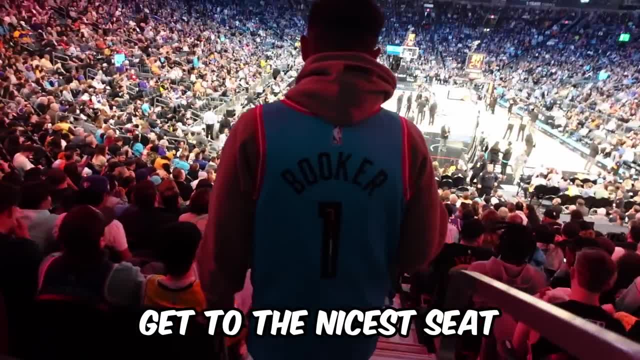 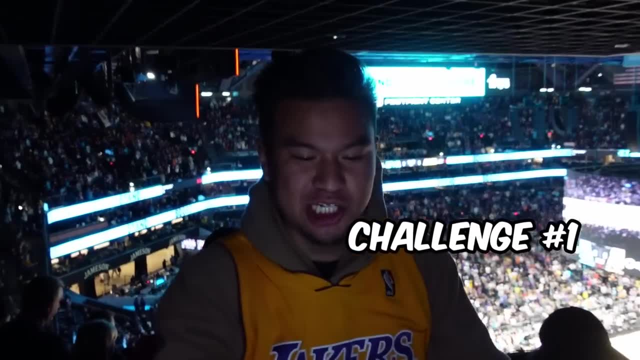 seating right behind the players. Our goal is to get to the nicest seat by the end of the fourth quarter, or the $1,500 tickets will go to waste. The tip-off has started and challenge one: Become a Suns fan. There's only one way to do that. I'm sorry, Lakers, And we're at the Enemies team store. 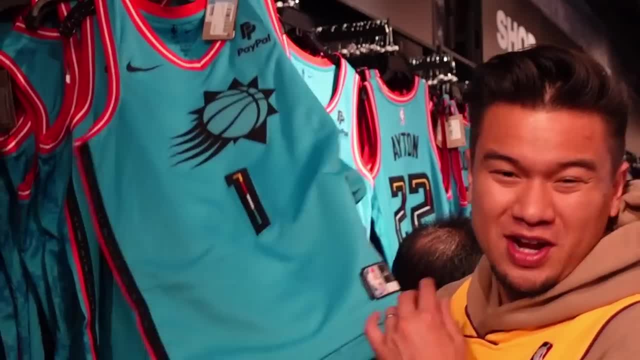 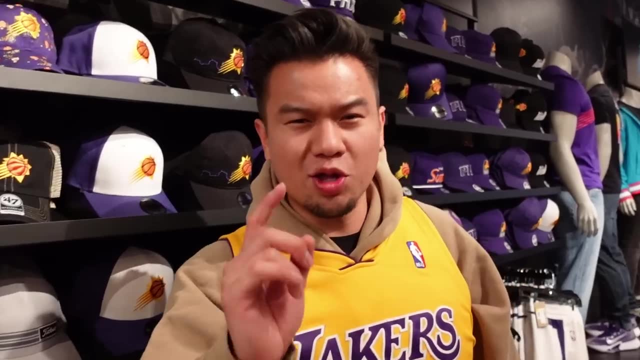 Let's go. They have these new blue colorways, Devin Booker, absolutely fire. They have the original the Valley jerseys, Chris Paul, and they even have the OG throwback Suns jersey. But there's only one right answer and I'm going with bam Devin Booker. We have unlocked our 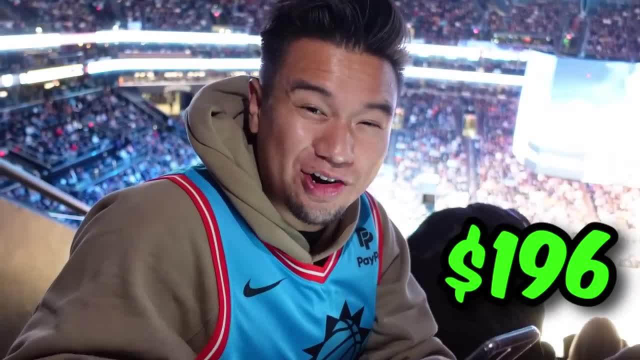 next ticket. They're in section 220.. These tickets cost $196.. And check out this view. Our next challenge is a challenge from one of the best teams in the world. Our next challenge is a challenge from one of the best teams in the world. Our next challenge is a challenge from. 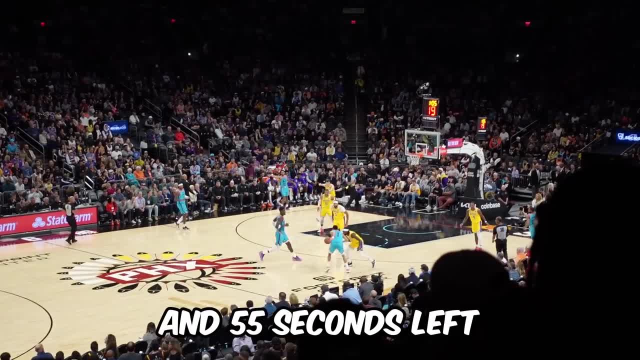 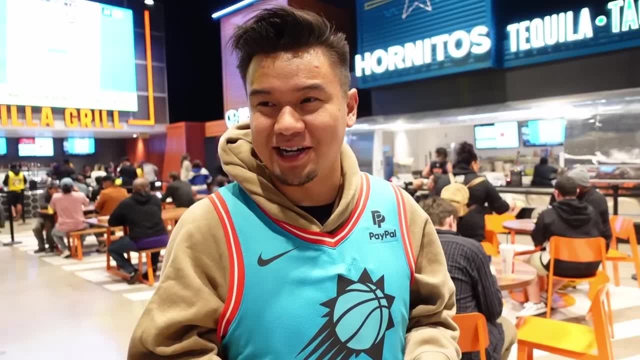 to an eating contest. It's the first quarter. There's two minutes and 55 seconds left. We got to go, So I have to find someone to challenge to a drinking or eating competition. That's the hardest part. I can't find anybody that wants to challenge me. Maybe I'll hold up a sign. 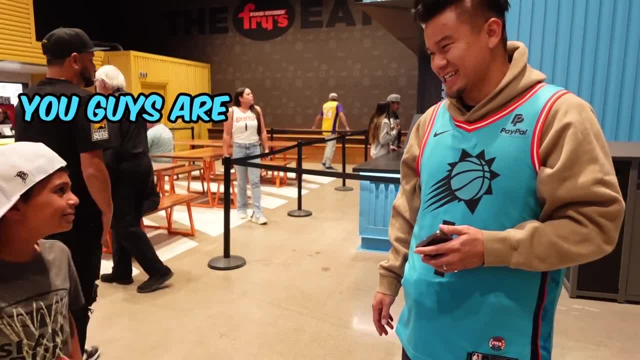 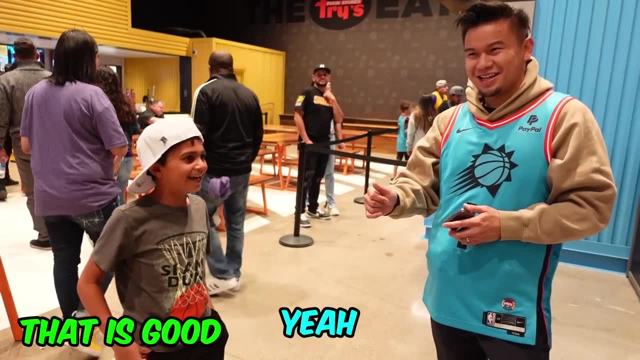 Yo, what's good, my man. You guys are making a video. Yeah, we are. Can I be in it? Do you want to challenge me to a food eating contest? Is that okay with your dad? Yeah, All right, We're going to get a cookie. What's your name, man? 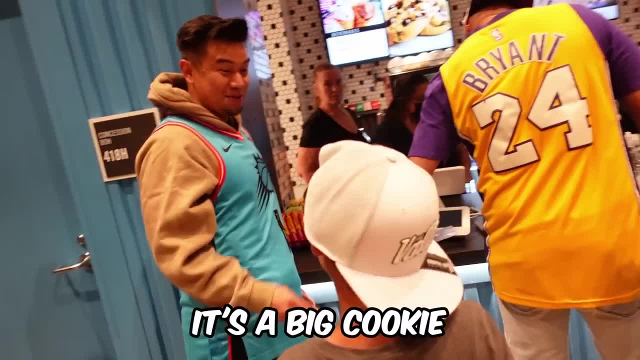 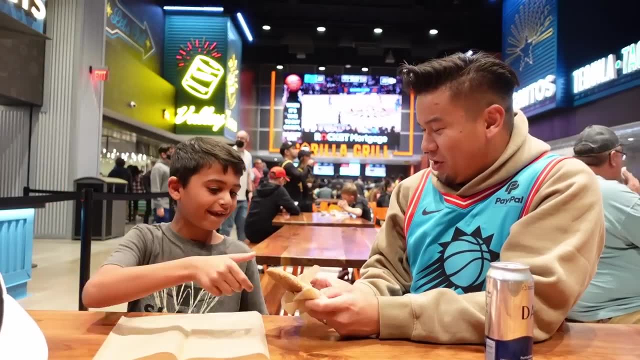 Noah, Can you eat a whole cookie or should we split it in half? Whatever, It's a big cookie. Okay, Jeff, really just challenged a kid right now. You see how big this cookie is. Yeah, And it's going to be a luck of the draw. Whatever breaks, that's yours. 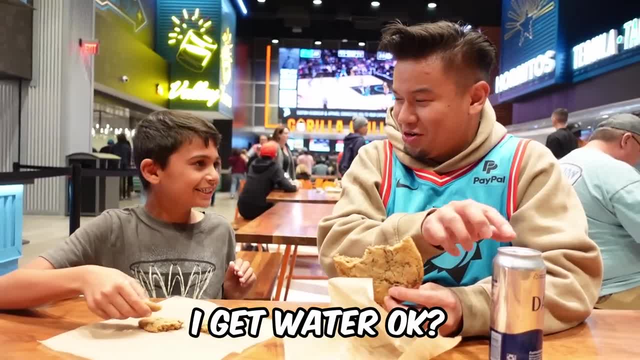 Show them your size. Okay, fair enough. Hey, Noah, I get water. okay, Is that okay? Yeah, So what's on the line is: if I beat Noah, I get to move on to my next seat. If Noah. 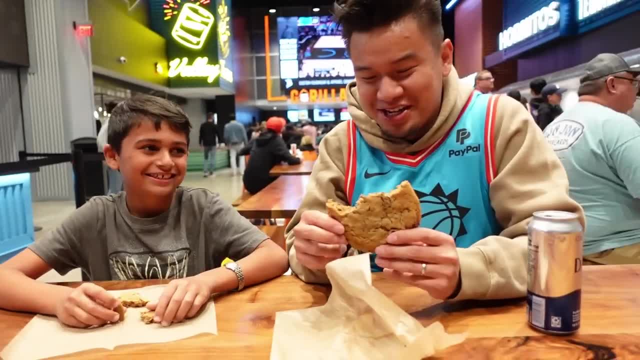 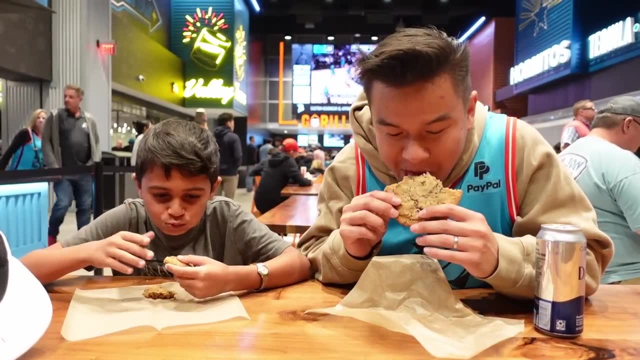 if you win, I'll give you $20, okay, I'm actually nervous. All right, Start when you're ready. Give us a countdown, Justin. Three, two, one go. Three, two, one go, One, two, one go. 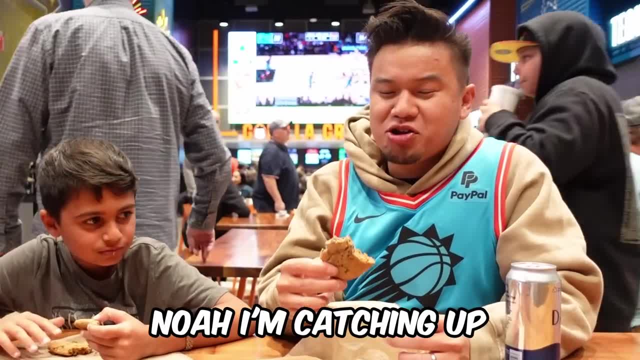 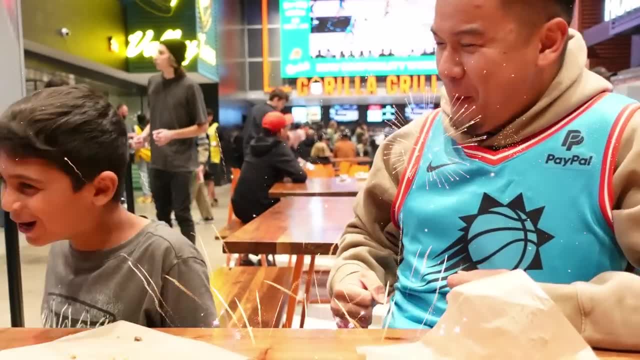 You surrender? No, No, that's enough. No, I'm going to show it's clean, Jeff. No, Ah, let's go. Good playing, Noah. I appreciate you, man. We're moving on to the next seat. 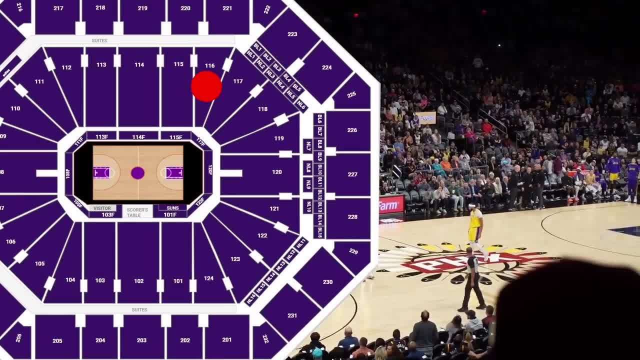 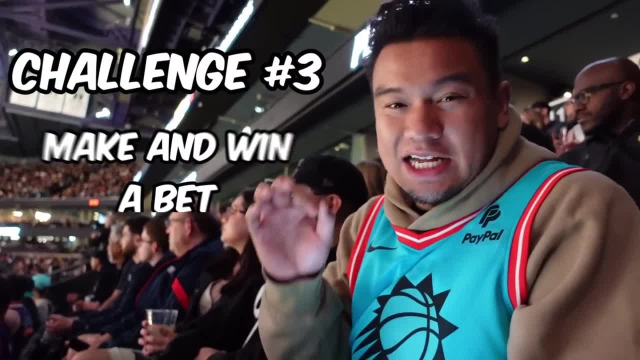 Let's check out these seats. These are row 116.. These seats cost $250.. Look at this view. We're way, way closer than before. Our next challenge to get to the next seat is to win a bet. We are now in the sports book. We've got to place a bet that's going to win. 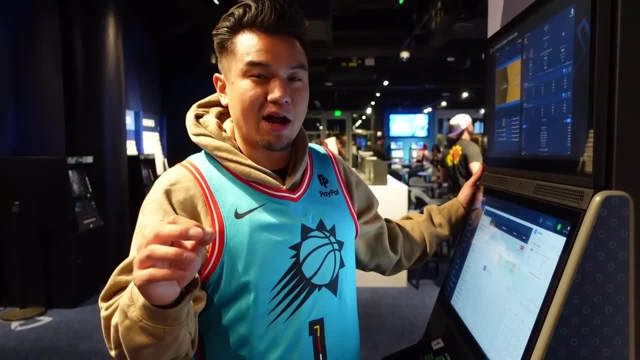 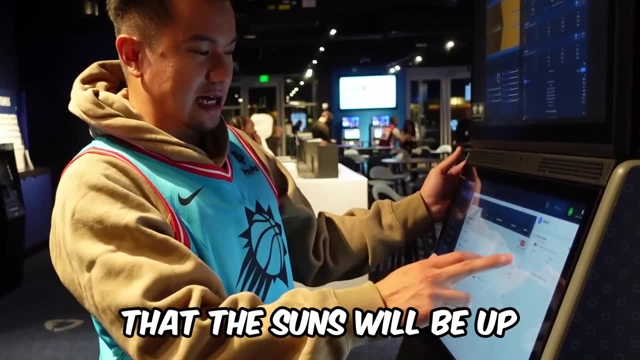 One bet only. I need this dug. So I'm placing a bet right now to either have the Lakers be up or the Suns be up at halftime. Lakers are down 10 points. I'm betting that the Suns will be up. I'm betting $20 to win $1.25.. The Suns are up by 10 and there's only four minutes left in the. 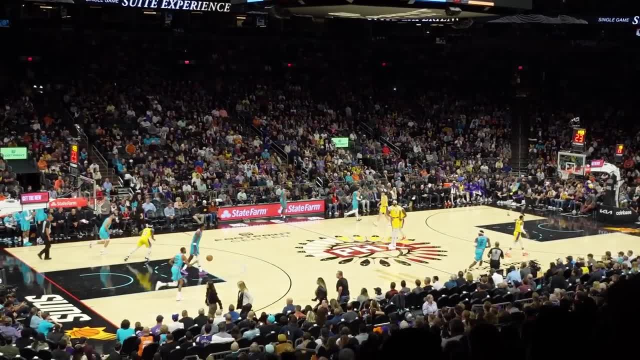 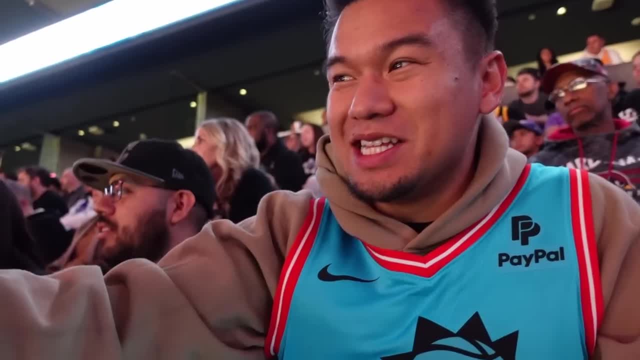 quarter. Let's go check it out. We are back in our seats. The game is tied, bro. The Sun- oh my goodness bro, What happened? We need the Suns to win or be up by halftime. The Suns are up by 10 and there's only four minutes left in the quarter. Let's go check it out. 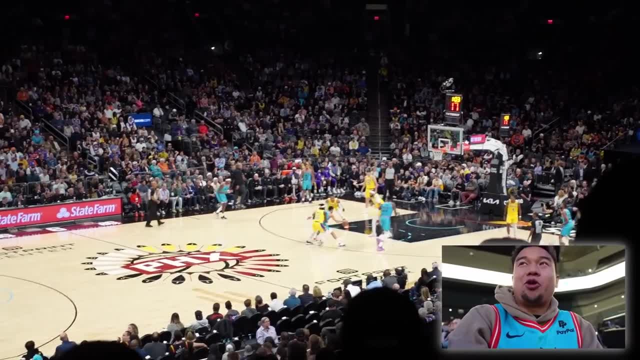 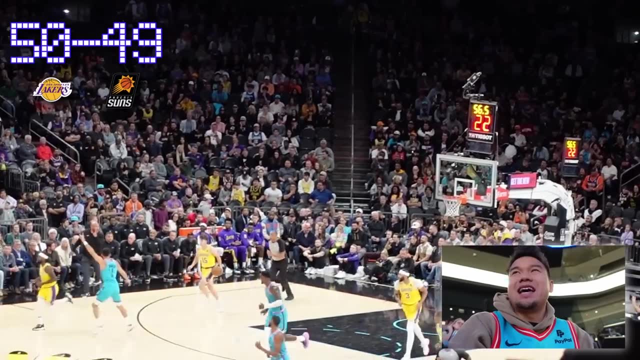 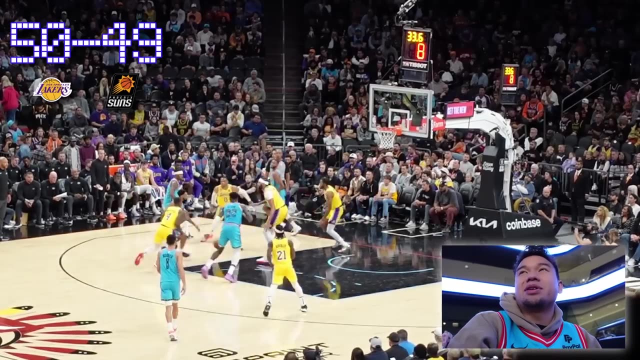 The score is now. Lakers are up one: 50 to 49, and Devin Booker passes Three-pointer. Oh, we needed that one, Bro. we should have betted on the Lakers. All right, we need a three-pointer right here. Go ahead, Cameron, Let's go, Let's go. 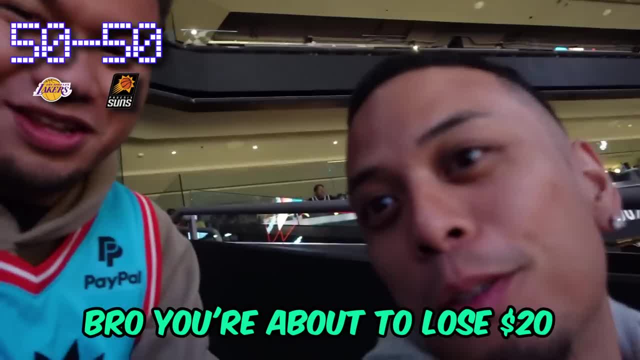 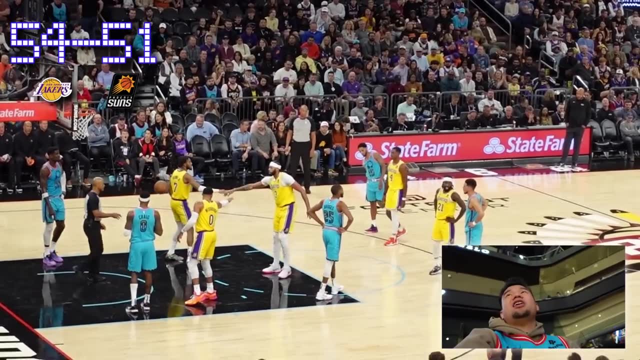 Rigged, bro? There's no way. it's not rigged, Bro. you're about to lose $20.. That's crazy. Three shots, That's crazy. Four is now 54 to 51.. The Suns are down by three. 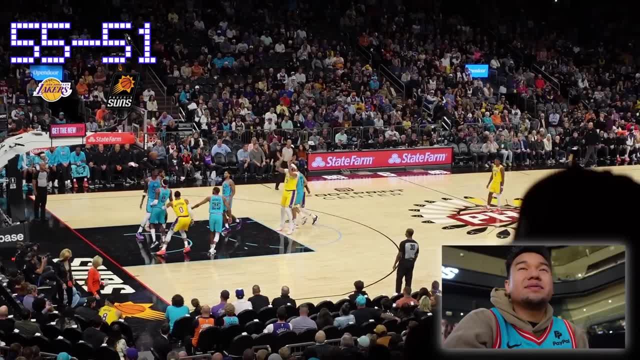 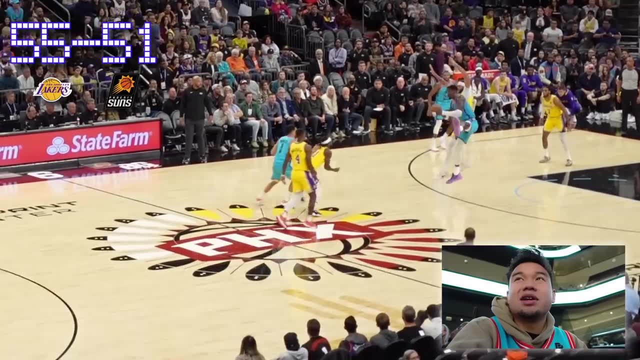 7.5 seconds left on the shot. Now the Suns are up by four 7.5 seconds left. It's a lock that we lost this bet. They can't even get the ball in, Devin Booker, Oh, Oh. 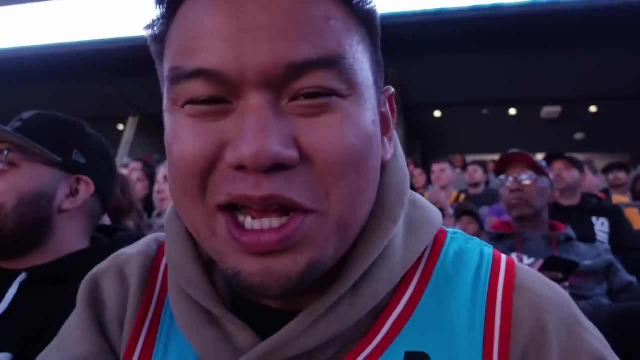 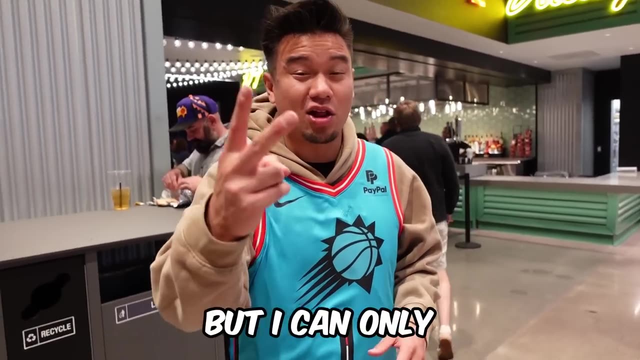 It's halftime and we lost our bet. If I can't complete the challenges, I can't go on to my next seat, but the NBA will send me another challenge if I request it. but I can only do this twice, Since I wasn't able to complete that challenge. 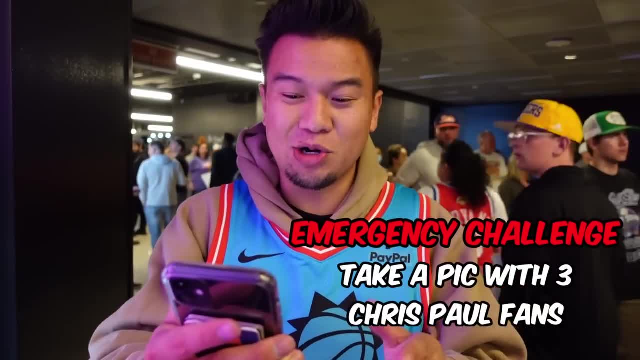 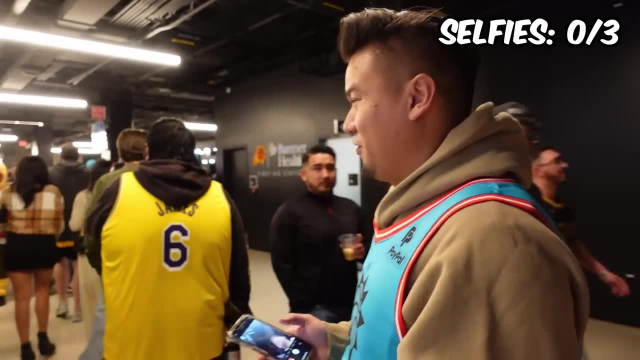 I requested an emergency challenge. Emergency challenge is to take a picture with three Chris Paul fans, So anybody that's wearing a Chris Paul jersey. I need to do this quick to move on to the next one. I don't know how to ask people for a picture. That's a weird thing to ask. 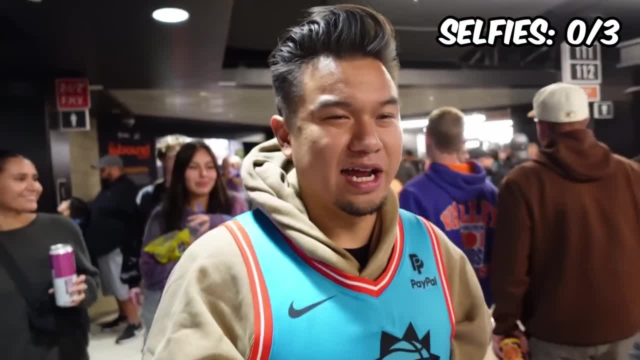 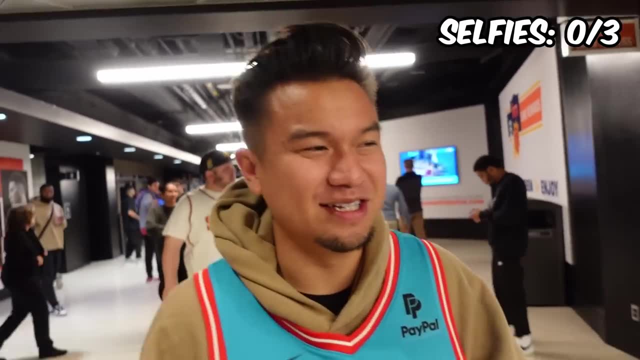 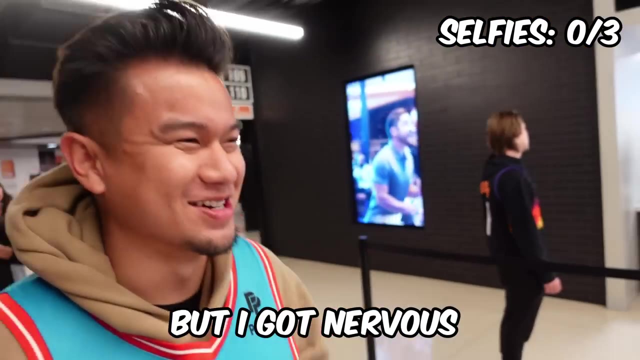 somebody Zero. you haven't seen a Chris Paul jersey? I have not seen a Chris Paul jersey. We took a whole lap already. I do not want to use both of my emergency challenges in one challenge. This is ridiculous. Oh, That's ah. I'm sorry. I felt my first Chris Paul and I got nervous. 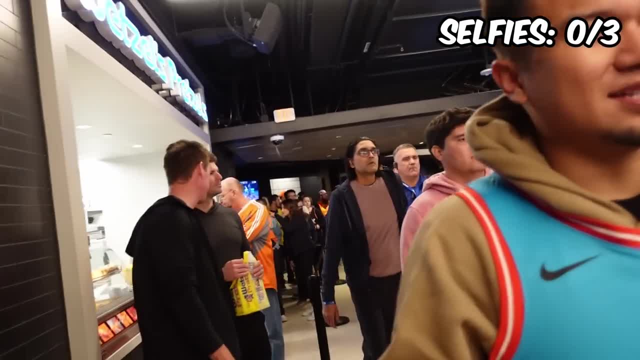 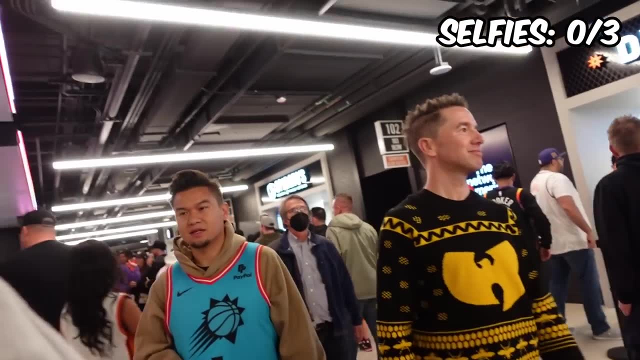 Dude, I might lose based off of this challenge. This is ridiculous right now. Justin, if you see anybody with a Chris Paul jersey, please let me know. Are you kidding me? Where, Where, Where, Where, Where, Where- Excuse me, Brody. 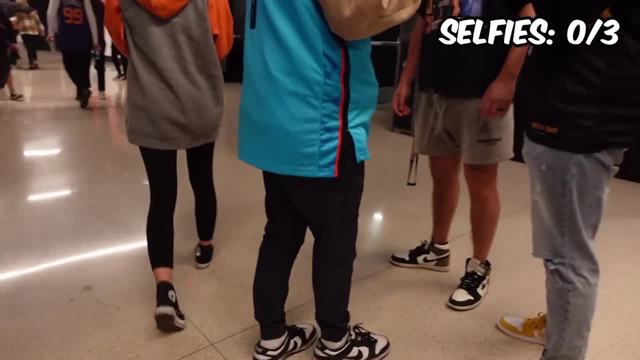 I'm so sorry to bother you. You are one of the only people here that have Chris Paul. Can I take a selfie with you real quick? Yeah, bro. Thank you so much, bro. I appreciate it. man. All right, one down, We need two more. 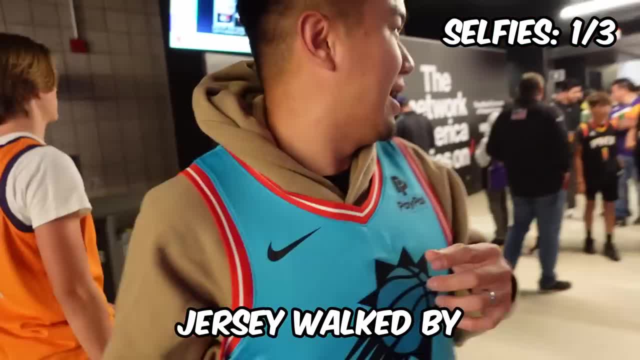 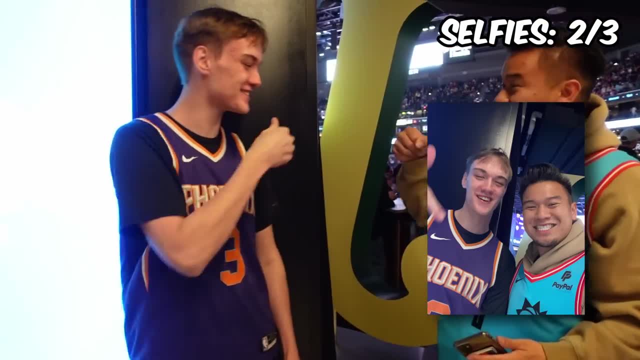 This is crazy. Another Chris Paul jersey walked by. Is that him? Yes, Hey, Brody, Can I take a selfie with you? Thank you so much bro. Go, Chris Paul. Yes, sir, Thank you so much bro. 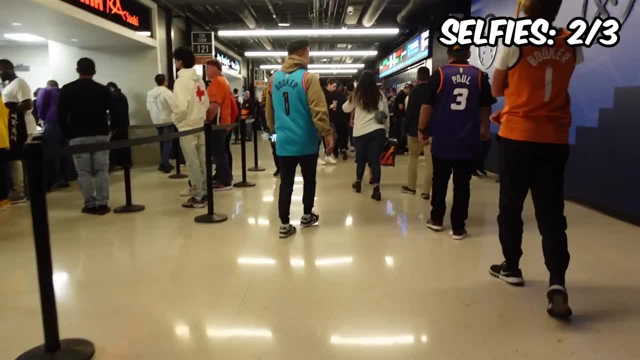 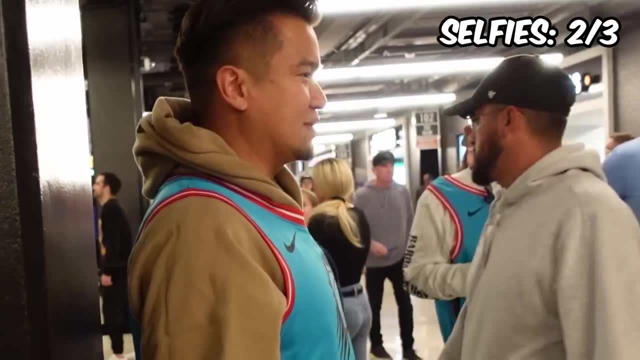 Oh, Oh, It looks kind of scary. That guy was ready to scrap bro. We need one more. Chris Paul, We're going to let the Chris Pauls come to us. Chris, Chris Paul, Your name's Chris Paul, Where That works. Do you mind if I take a selfie with you for the challenge? 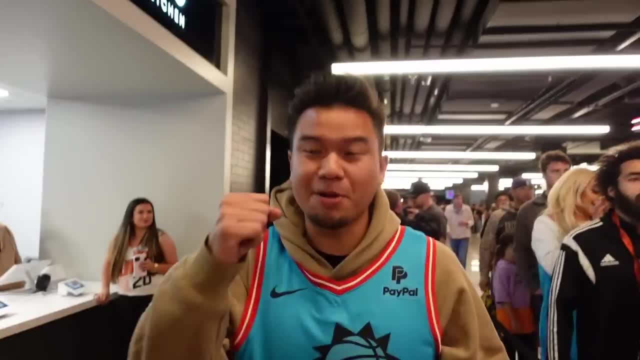 Let's do it. Thank you so much, bro. I appreciate you, man. All right, we completed the challenge. Let's go Going on to our next seat and let's check it out. We have moved on to our fourth seat. 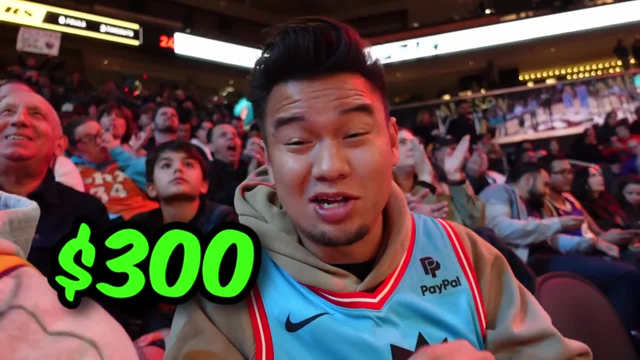 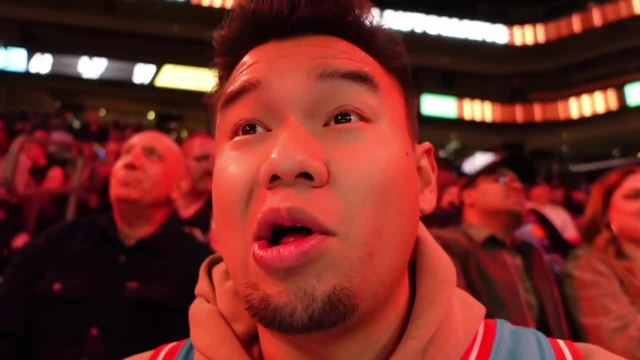 row 121.. And these tickets cost us $300.. Check out the view. We're going to enjoy the game a little bit, but I'm going to read our next challenge to keep it in mind. We are so close. It is the third quarter. There's eight minutes and 37 seconds left. 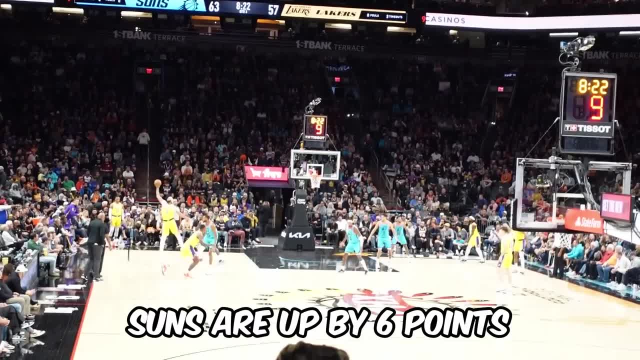 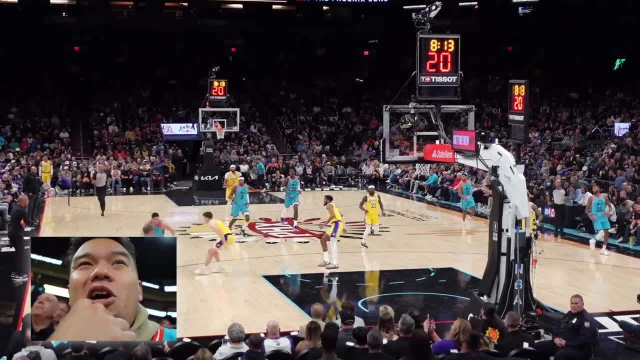 And we still got two challenges to complete to get to the best seat. Suns are up by six points All of a sudden. Oh, Suns, with the steal Devin Booker driving down the lane. Oh, Finished with the left-hand lane, Let's go All right. What are we doing, bro? I know we want to. 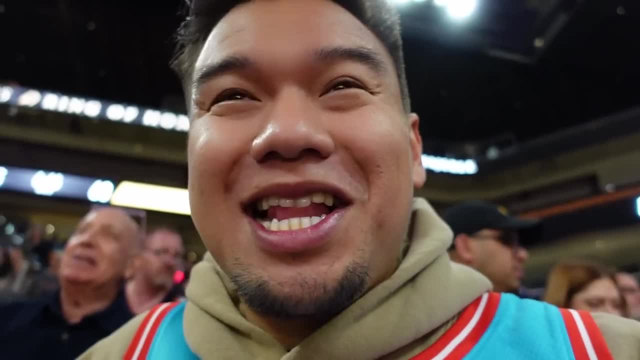 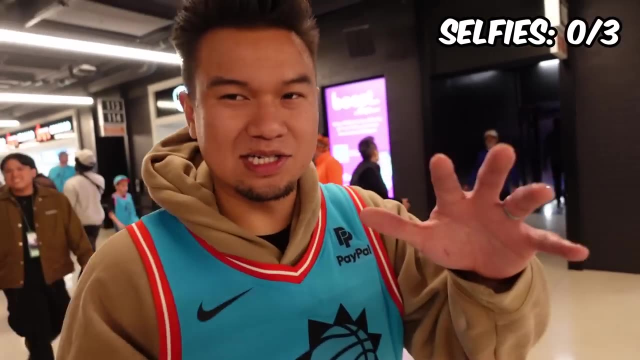 enjoy the game, but we got to go do the challenges. We just want to watch the game. We got to get to the last seat. I have to take a picture with three away fans. Lakers Nation for life. I'm waiting for this guy to come out. There's also a guy in the shop right now. 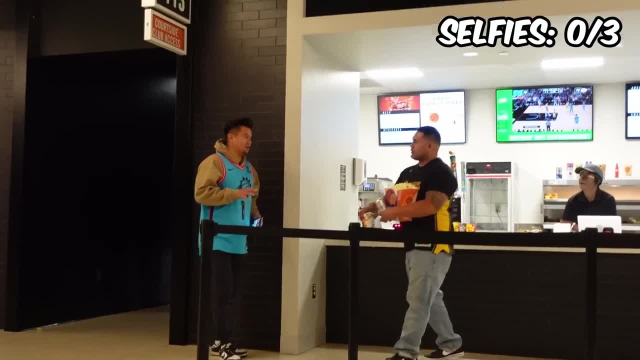 This is not that easy. Hey, buddy, I'm so sorry to bother you. Do you think I could take a selfie with you? But thank you so much, man, Appreciate it. One down, two more to go. People are so nice. 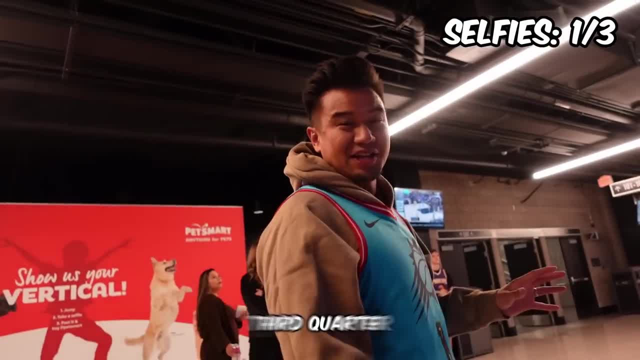 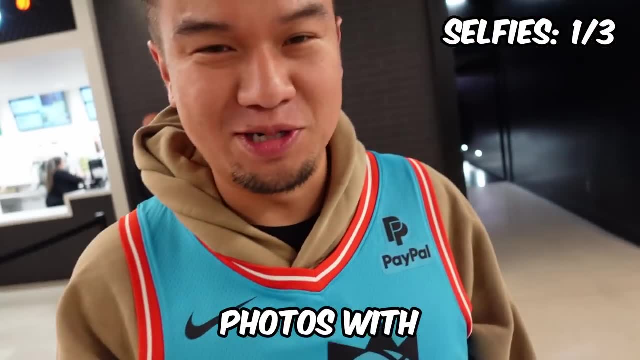 No one has rejected a photo with me yet. I'd be sussed out. Oh, it's the end of the third quarter. We really need to go. We might fail this challenge because of my lack of ability to take photos with away fans right now. Yes, very empty, Hey, buddy. 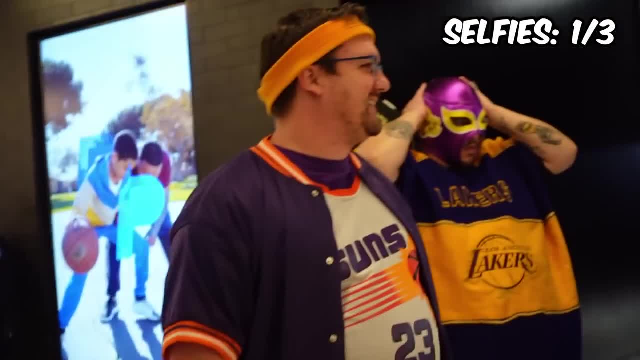 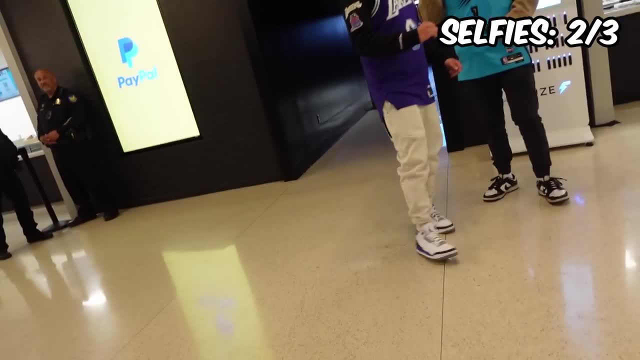 Can I take a picture with you by chance? Yes, Thank you so much. I love the fit. Appreciate it, man. Thank you so much. Thank you. I'm doing a challenge right now where I have to take a picture with three Lakers fans. 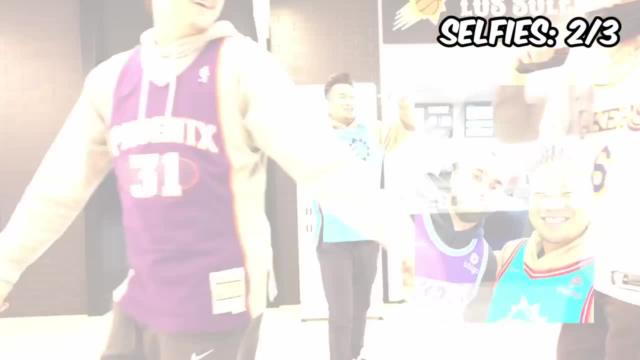 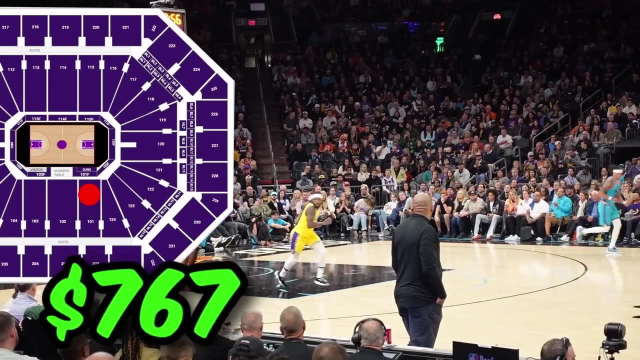 You're my last one and I'm done with the challenge. Thank you, Thank you, Thank you, Let's go. All of a sudden, there's so many Lakers fans. We just unlocked our next seat. Let's go. All right, These are definitely the best seats yet. My next challenge: to get to the next seat. 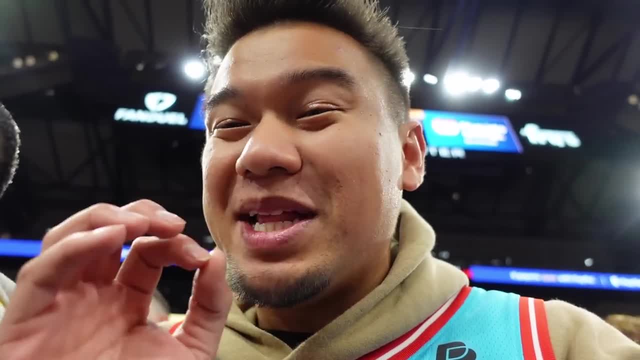 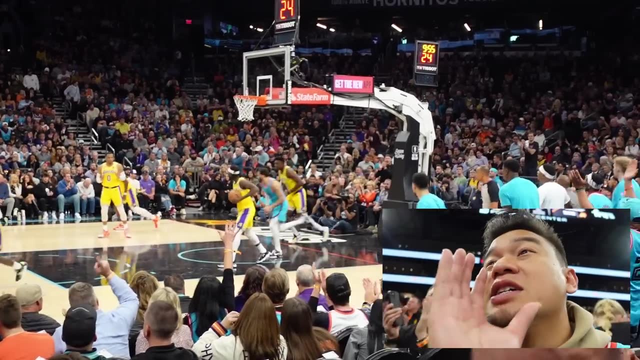 is get Devin Booker's attention and yell his name. So I'm going to at least yell my name and tell the NBA that I got his attention. Devin, All right, He didn't look. I'm going to try again. Devin Devin, He stood up. He stood up. Devin, All right, This is not working, Since we couldn't. 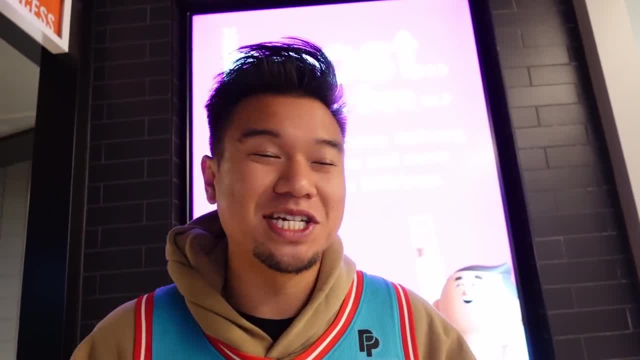 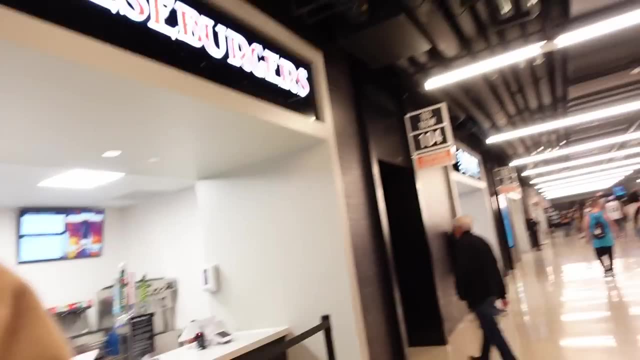 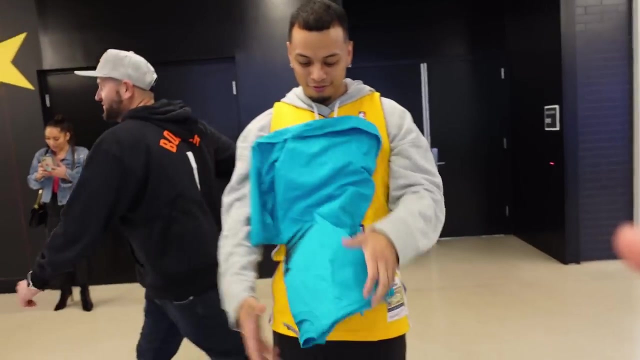 get Devin Booker's attention. we requested one last emergency challenge. A sun stand just came up to Justin and gave him a Phoenix Sun shirt, because the Lakers are losing right now. I said that's actually fire, bro. All right, The last challenge is to trade the shirt for another sun's gear. It could be for anything. 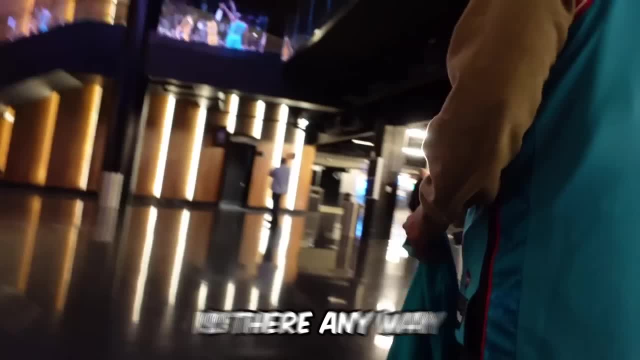 This might be hard, but we'll see. I'm so sorry to bother you. Is there any way I could trade you this shirt for that hand? Okay, Thank you so much. I appreciate it. We got the trade. Let's go All.